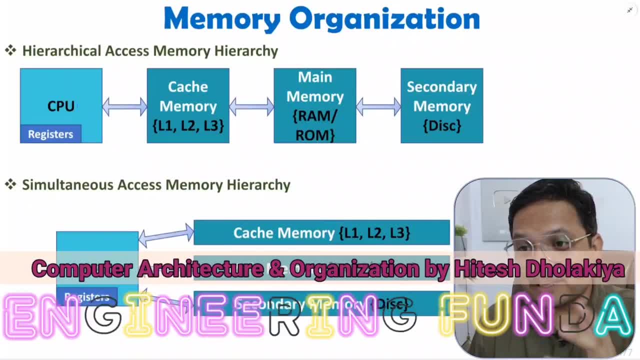 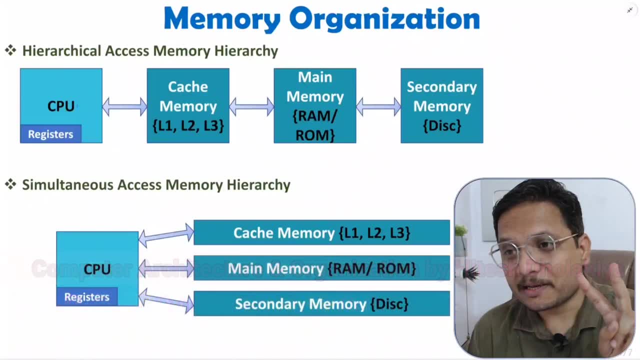 Hello friends, welcome to Engineering Funda family. In this video I am going to explain you memory organization in computer Basically. there are two ways by which memory can be organized with computer. One is hierarchical access memory hierarchy. The second is simultaneous access memory hierarchy. Usually you will be observing hierarchical access memory hierarchy that is being utilized with majority of computer systems. 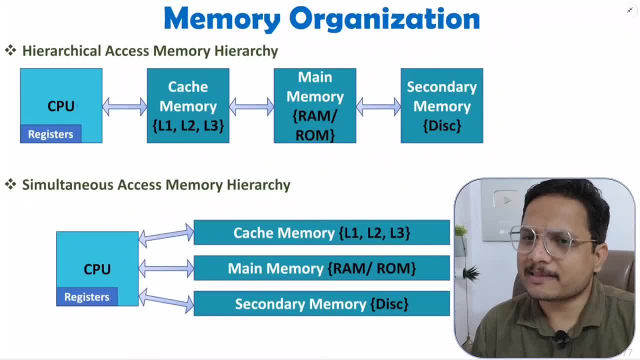 There are very few systems which is using simultaneous access memory hierarchy. Why? The reason is there are some advantages of hierarchical access memory hierarchy. Simply the major advantage is what? The major advantage is access speed, As if you have hierarchical access memory hierarchy then that execution speed of program that will be way faster compared to simultaneous access memory hierarchy In my computer. I am having hierarchical access memory hierarchy with my computer. 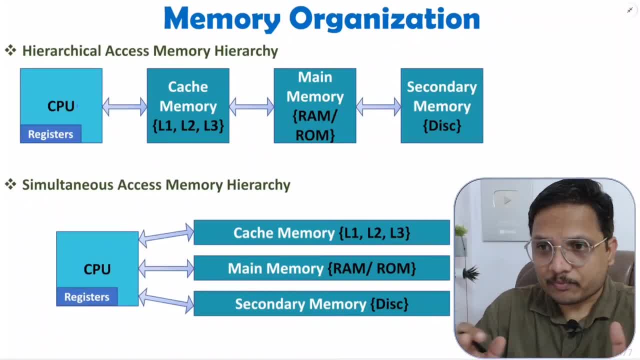 In this video I will show you how exactly that structure is there with entire memory organization with my computer. Let us try to understand first how basically these memories are organized. So you see, in hierarchical access memory hierarchy this is CPU. Within CPU there are resistors. That is also memory that you can say It is having size, which is there in terms of few kilobytes, Right, And if I say execution speed is 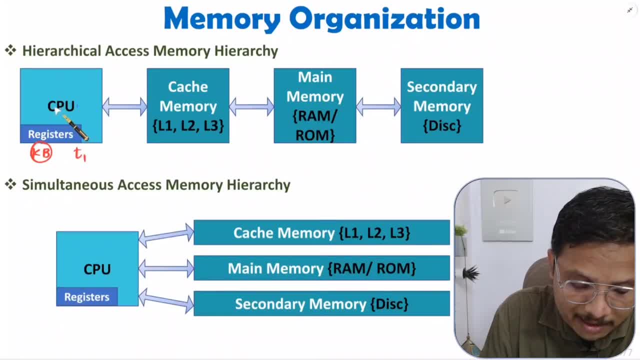 time that is T1, then that is what fastest which is there with CPU. Fastest means what? That execution time will be lowest compared to other memory. When we talk about cache memory, that is there in terms of few MBs. And if I say execution time that is T2, then that is bit higher compared to T1.. Why? The reason is this: cache memory is bit slower compared to resistor, But that cache memory that is way faster compared to this main memory. 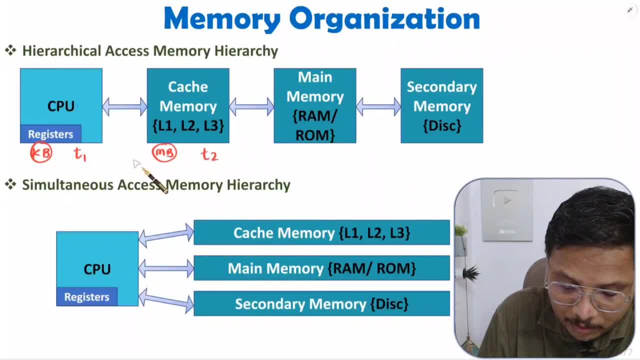 And secondary memory. So you can say execution time T2, that will be bit higher compared to T1, which is there with resistors, But execution time, if I say that is T3, with this main memory which is RAM and ROM. So that execution time that will be bit more compared to cache memory over here And you will be observing this RAM, which is main memory, that will be there in terms of few gigabytes. I will show you example of my computer So you will be having 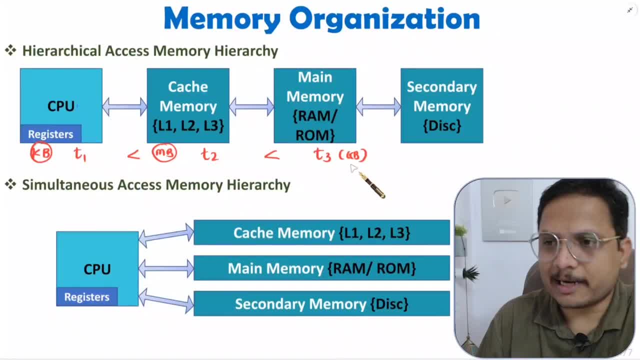 fair enough idea about how exactly these memories are there, Right? Let us try to understand first how exactly these memory are structured over here with CPU- See secondary memory. usually that is referred as disk. If I say execution time, that is T4.. So obviously that will be greater compared to execution time which is there with this other memories And you will be observing- that is there in terms of hundreds of gigabytes. You can say it may be there in terms of 1 terabyte, 2 terabytes nowadays, in 2023. 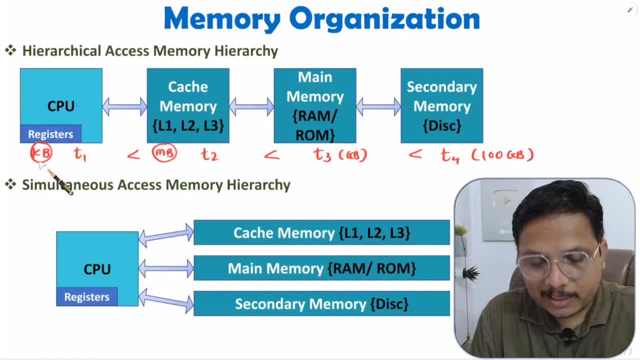 But if you observe over here, resistors are there in terms of few kilobytes. Cache memory- that is there in terms of few MB, This main memory, that is there in terms of few gigabytes. You can say you may be having 8 gigabytes or 16 gigabytes of RAM with your computer And secondary memory that will be there in terms of hundreds of gigabytes. If you observe execution time, then you see, as you go closer to CPU, execution time is decreasing. Execution time is decreasing means what? 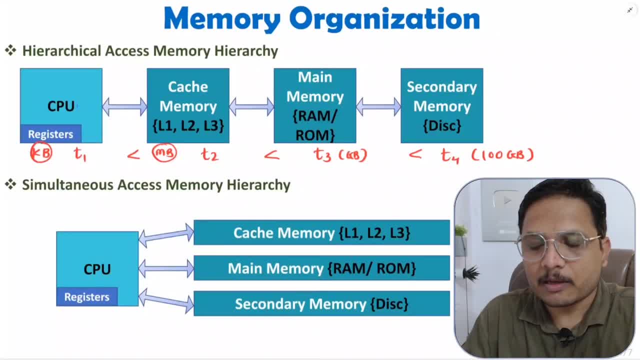 Here access speed. that is increasing. So obviously whenever you access any program, at that time that program should be very closer to CPU. Like, for example, CPU is accessing one program Right, So as if that program is there with the nearest memory, which is cache memory. in that case that execution speed will be highest. So let me give you an example how exactly CPU is executing program. See, whenever CPU wants to execute any program, it will be generating a lot of RAM. 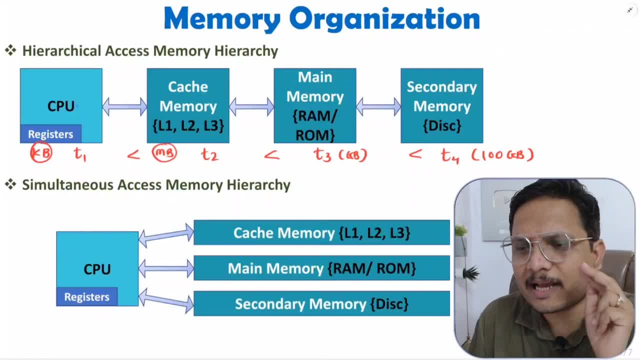 It will be generating address first. Always, CPU generates address of program to be executed right now. Let us say CPU have generated one address for particular program, Right? So what will happen? CPU will see whether that program is available in cache memory or not. If it is available, then it will directly access over here. But if it is not available, in that case that program that will get mapped at main memory, which is RAM. 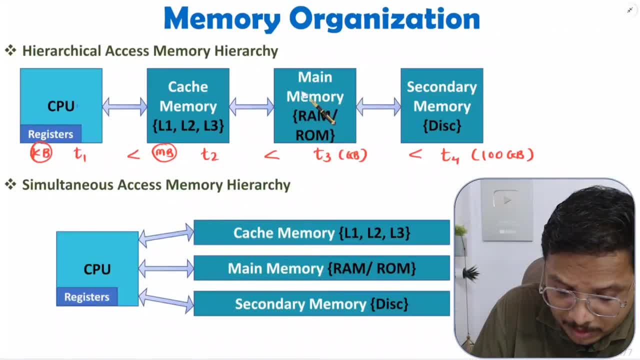 Now, as if it is available in main memory, then that program that will get transferred in cache memory first, and then CPU will access it, Right. But as if that is not available in main memory, then obviously it must be there inside secondary storage. And as if it is available in secondary storage, it will get copied inside RAM. From RAM it will get copied inside cache memory and then CPU will access it Right. Why that is happening? The reason is, my dear students, 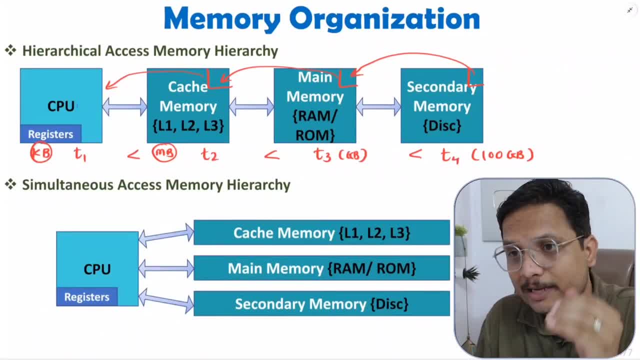 here you will be observing access time that is lowest with cache memory. So here, as if that program is not copied over here, then CPU will be accessing that program with secondary memory with more time means access speed will decrease over here. So in hierarchical access memory hierarchy CPU doesn't communicate directly with secondary memory. What it does is whatever address is being generated over here that should be copied over here. 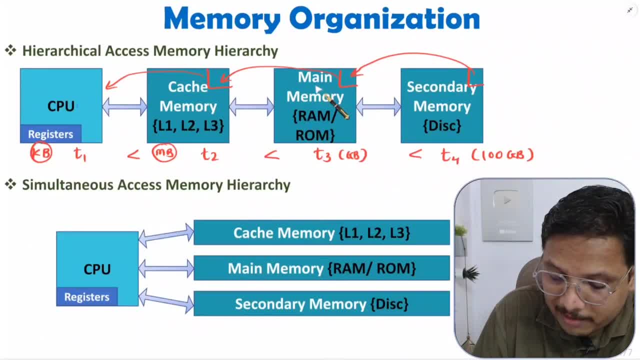 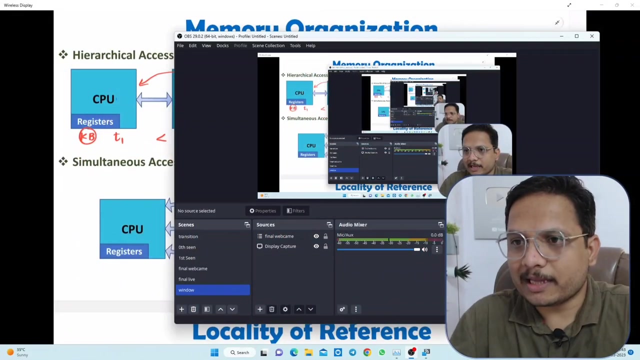 Inside cache. if it is not copied, then it will take it from main memory. If it is not available in main memory, then main memory will take it from secondary storage. From main memory again it will get copied inside cache And then from cache CPU will access those addresses which is generated for particular program. Right, Let me show you how exactly structure is there with my computer, So you will be having fair enough idea about how we can have that execution. So if you observe 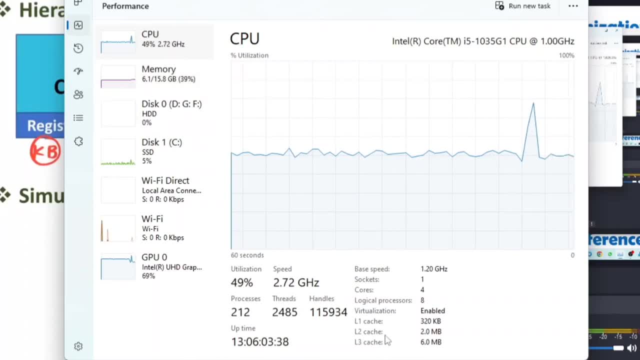 that task manager window of my computer, then you can observe here I'm having three level cache memory which is there within my computer: L1 cache, L2 cache and L3 cache. L1 cache is having size of 320 KB, L2 cache that is having size of 2 MB And L3 cache that is there in size of 6 MB. Right, So three level cache memory is there which is there with my computer. So here what I have done was, if you observe here, 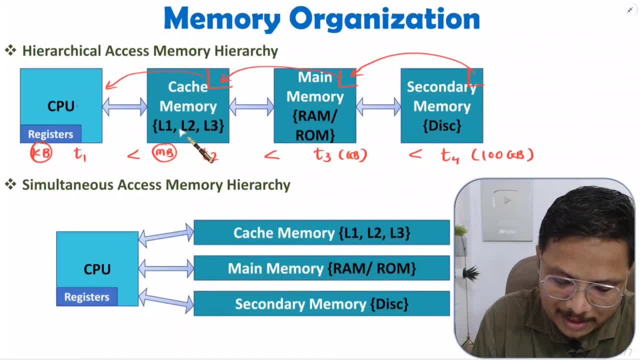 i have told you like i'm having cache memory, so there will be multiple levels, right? so here multiple levels are there. so l1, that is the nearest level which is there with cpu, from there l2 is there and apart from there there will be l3, right, so program that will get copied. 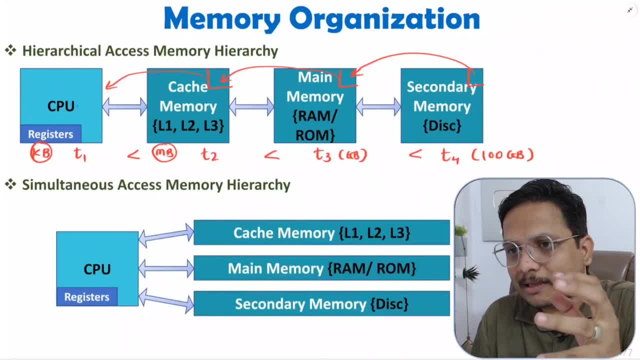 level wise and nearest level, that is l1, that will be communicating with cpu directly, right here, my dear students, in hierarchical memory axis, what will happen is like whatever program that is available in cache that is getting executed very fast. let me give you one example. for example, if i say that main memory is having time t3, right, then you will be observing that. 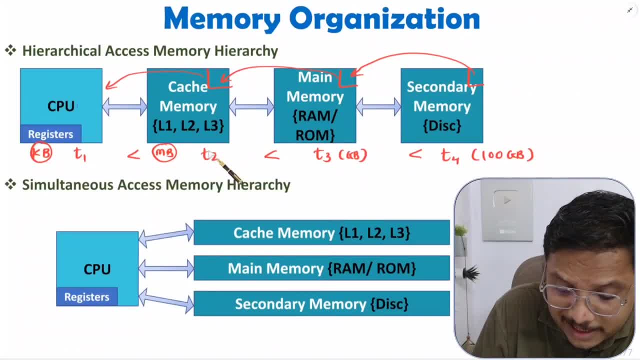 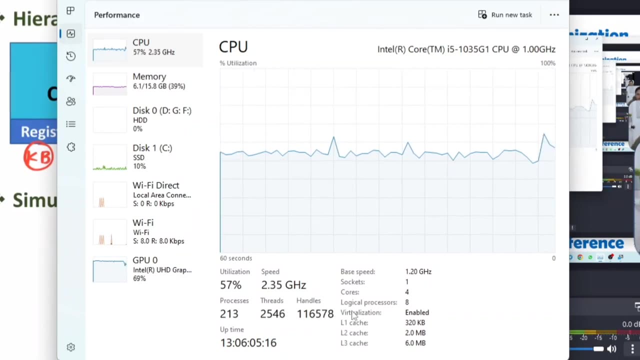 cache memory that will be taking 10 times least time compared to main memory, which is ram. right again, let me show you how exactly structure of memory is there with my computer. so here see, regarding cache, i have told you already now, if you observe this memory which 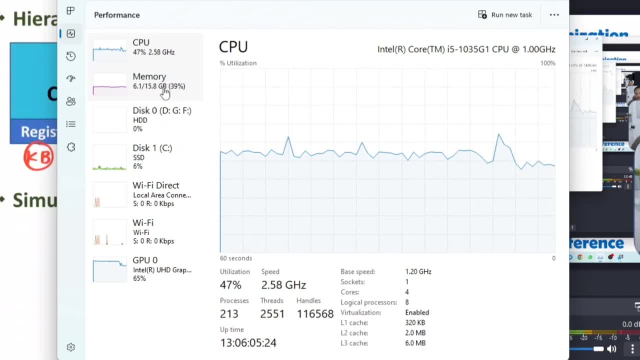 is written over here. that is main memory, that is ram of my computer. so that is having size of 16 gb. i have already told you that ram will be having size in terms of few gbs. after that, secondary storage is there, which is disk in my computer. there are two types of disks. one is hdd disk. 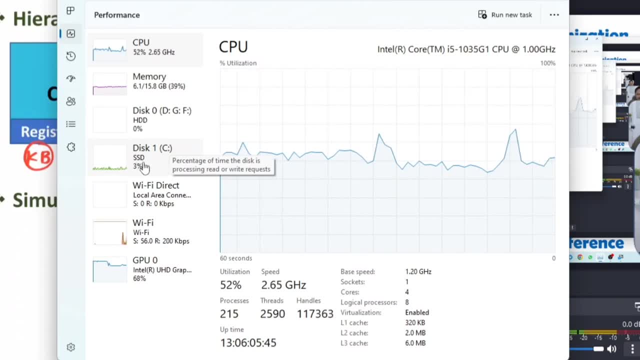 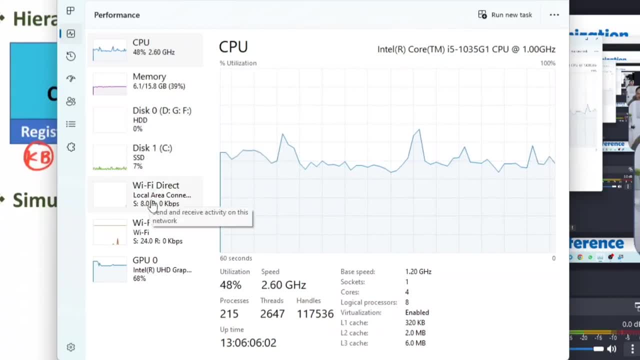 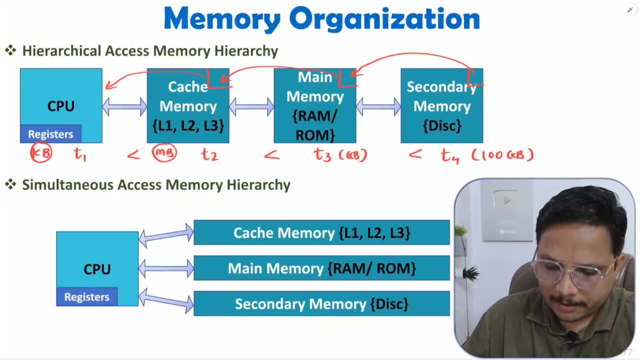 with my computer that is referred as secondary storage. so that is how complete memory organization which is there with my computer. Now let us try to understand all those things over here. so in hierarchical axis memory hierarchy, CPU will be executing programs from cache memory only. so if program is available. 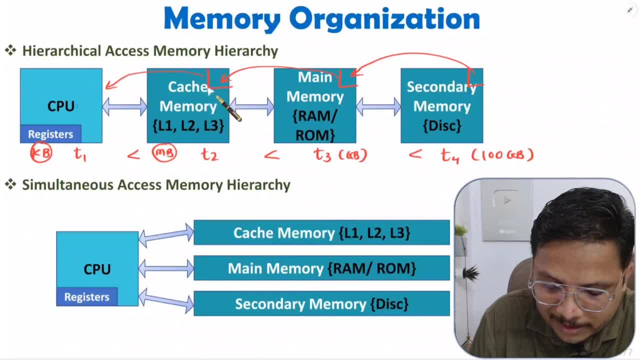 with cache, then it will directly communicate. if it is not, then it will take it from RAM, and if it is not available in RAM, then it has to be there inside secondary storage and at last CPU will be communicating with cache memory. only right, that is how things are. 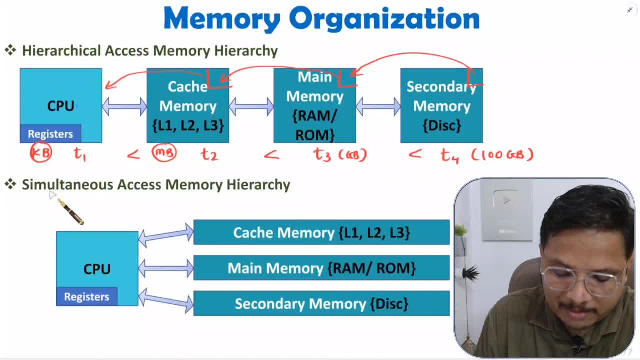 happening with hierarchical axis. Let me explain you: how simultaneous axis is there? so in simultaneous axis, my dear students, all the memories can communicate with CPU. so here see access time and all those things that I have already discussed. right? so what will happen is like whenever: 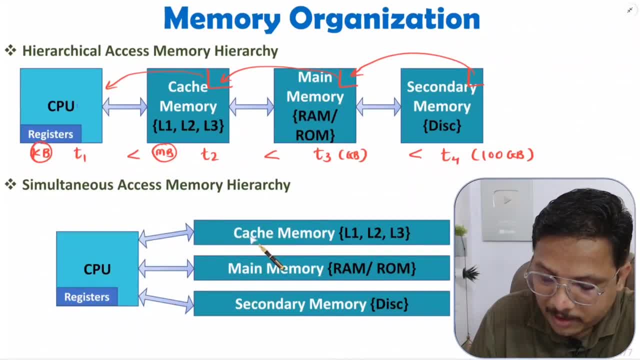 CPU wants to execute any program, first it will search inside cache memory. if it is available in cache, then it will access that program directly inside CPU. but if it is not available inside cache memory, then what will happen? it will search it inside main. 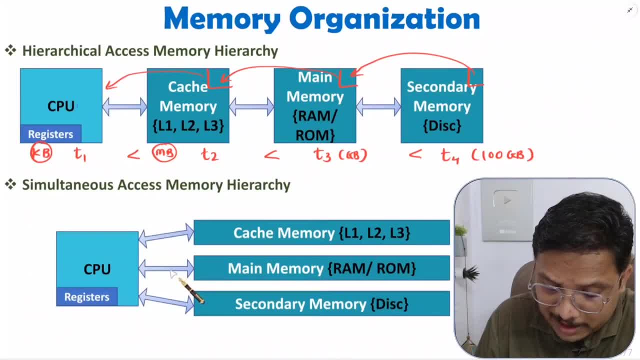 memory. that could be RAM or ROM. If it is not available inside RAM or ROM, then it will search it inside secondary storage memory, which is disk. so you will be observing whenever CPU is accessing program from secondary memory, at that time that execution speed will be very slow, as if CPU is accessing program. 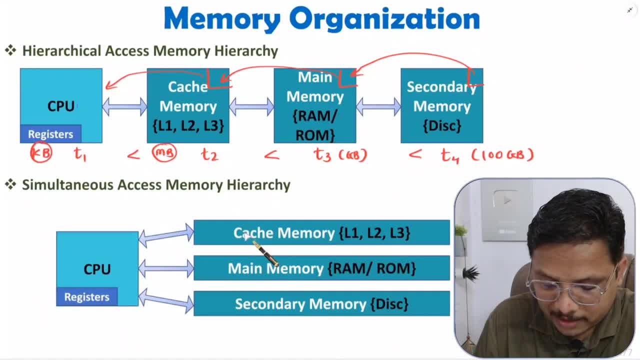 from cache memory. in this situation obviously that speed will be fast, but as if CPU is not accessing memory which is cache memory, in that case, with this type of memory hierarchy, that execution speed will be very slow. So usually you will be observing, in majority of system hierarchical access memory is there. 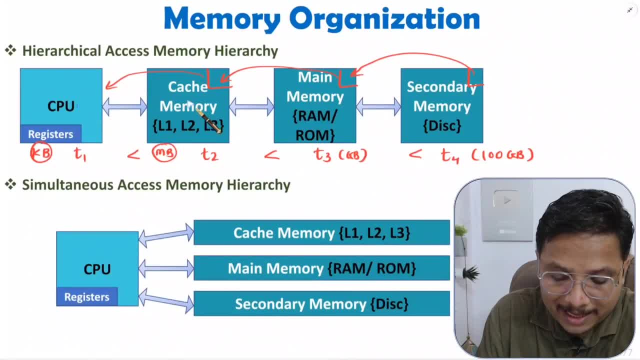 in which that CPU will be accessing programs via cache memory only. if program is not available inside cache, then it will copy it from RAM. if it is not available inside RAM, then it will copy it from secondary storage. so hierarchical access will be there at last, as if program. 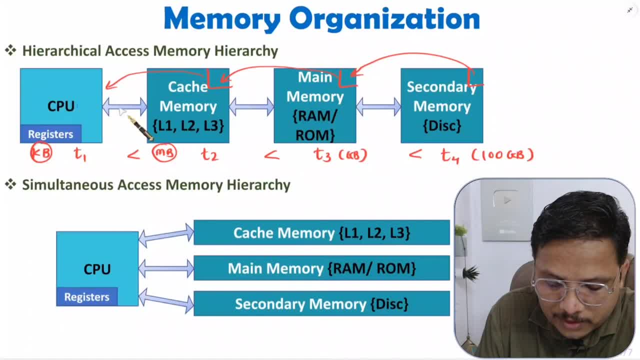 is available in cache memory, then you will be observing that execution speed that will be very fast. So that is how basic memory organization that will be there with majority of computers. My dear students, this is just introduction. in next coming videos I am going to explain. 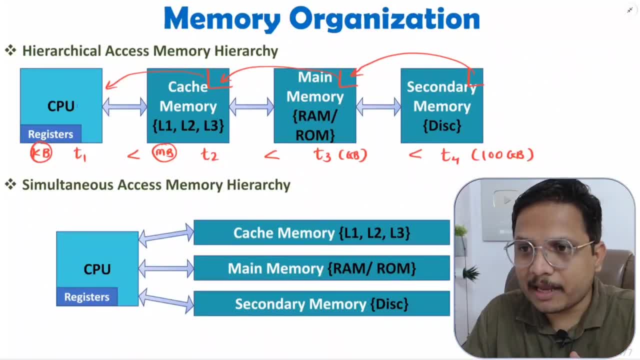 you how exactly memory mapping will happen within cache memory, how we can have a calculation of access time during execution of program. so all the basics, like locality of reference, how exactly locality of reference is happening, everything that I am going to cover in great 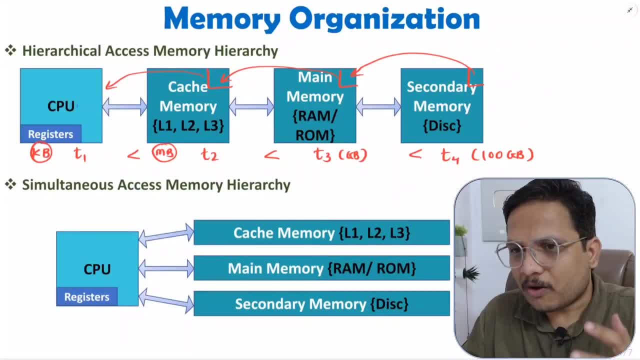 detail in future programs. So stay tuned with this playlist of computer organization and architecture. if anything that you would like to share it with me, please note it down in the comment box. I will be happy to help you. thank you so much for watching this video.